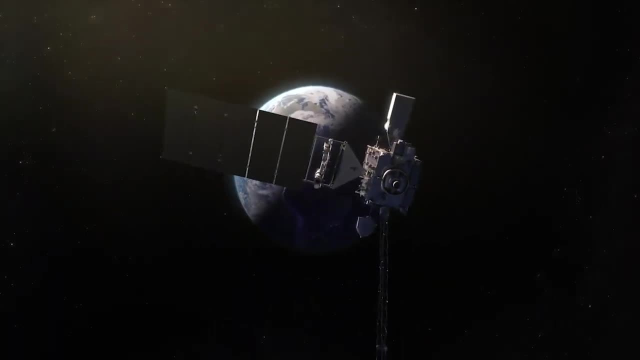 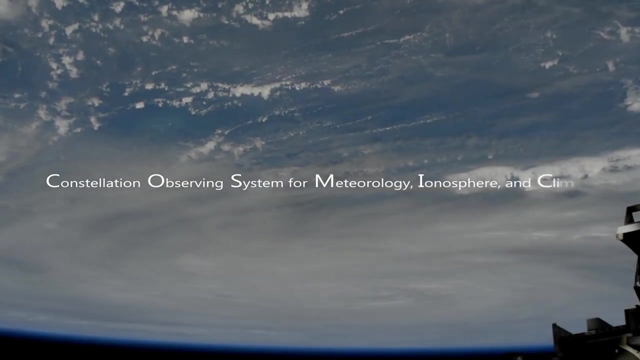 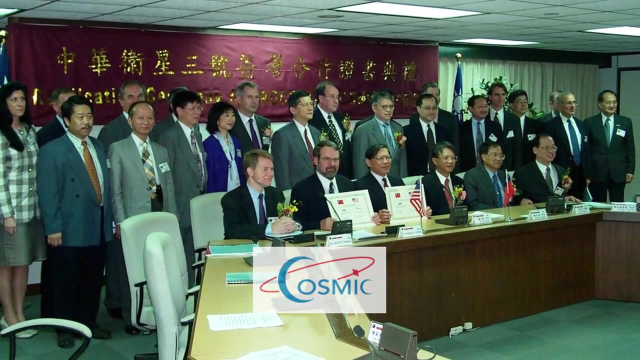 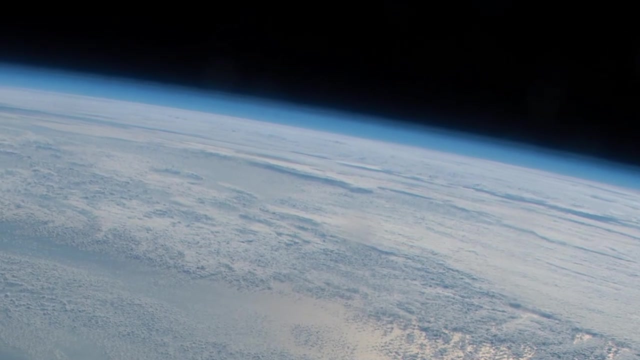 Satellites orbiting in space around Earth help scientists forecast when and where storms will happen. In 2006,, a new group of satellites called COSMIC was launched by the United States and Taiwan. COSMIC looks across Earth's atmosphere to provide important information to help with weather forecasting. 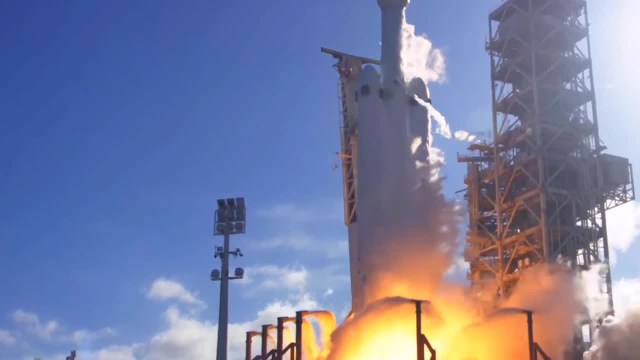 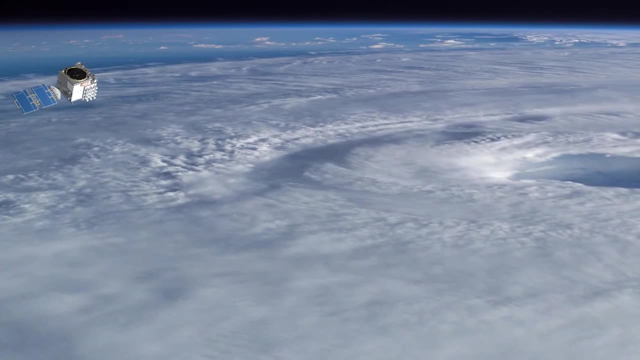 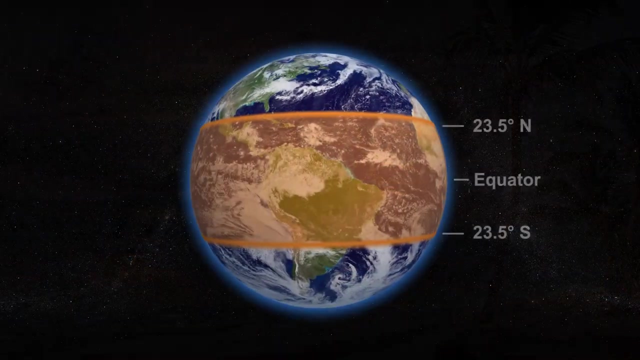 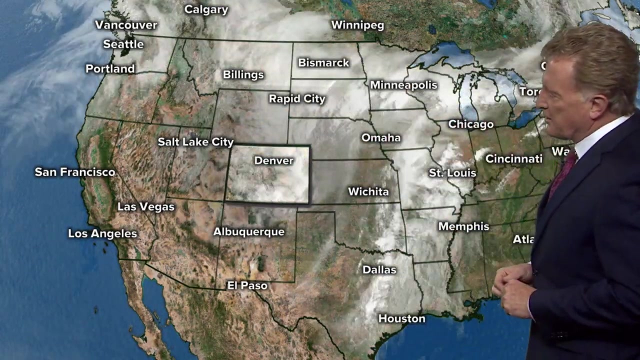 Three, two, one And zero and liftoff. And now a new, more advanced system called COSMIC-2 provides even more information which will improve storm forecasting, especially in warm tropical areas near the equator. Just beautiful structure on this storm as it's swirling across the central part of the country. 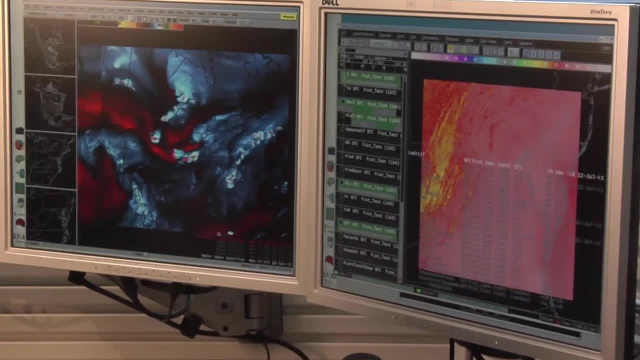 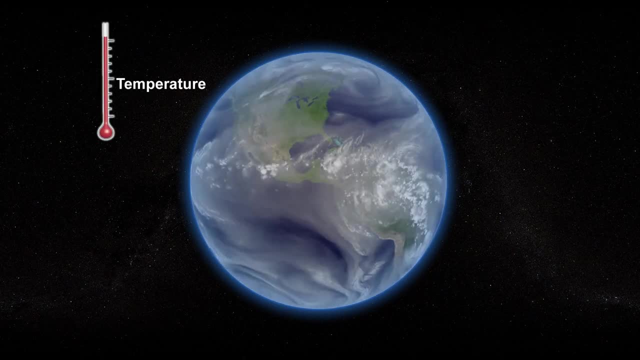 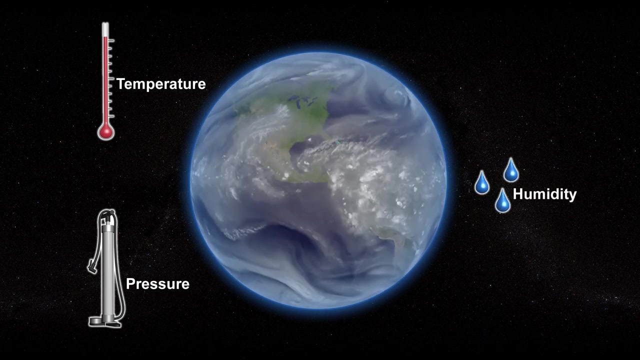 To make accurate weather forecasts, meteorologists and other scientists first need to know three things about the atmosphere: The temperature, how warm the air is. the air pressure, how compressed the air is at any one spot. and the humidity: how much water or moisture is in the air. 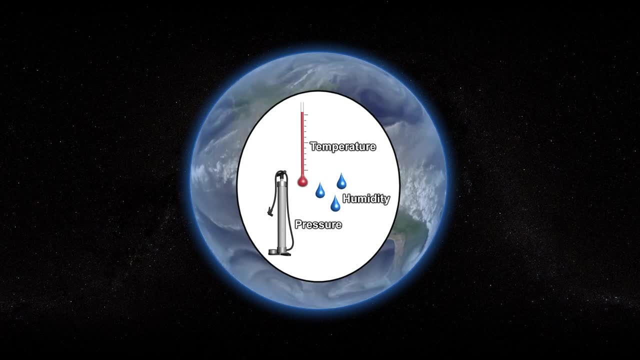 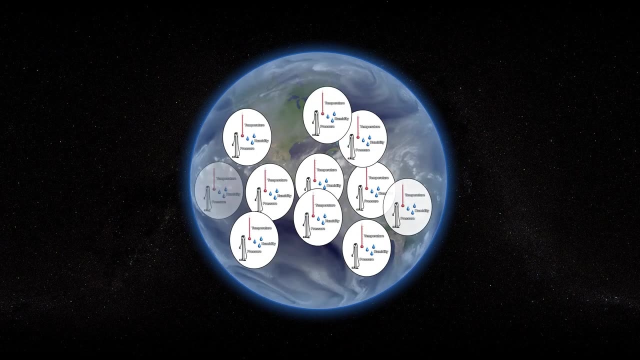 They need to know how these three things vary, at different altitudes or heights from Earth's surface and for as many locations on the globe as possible, Because what happens in one place affects the weather in other places. How can COSMIC-2 see these things? 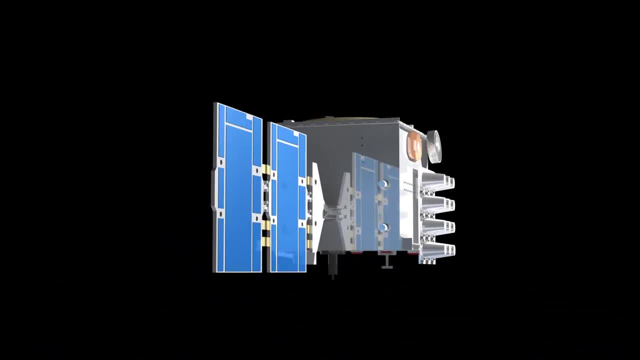 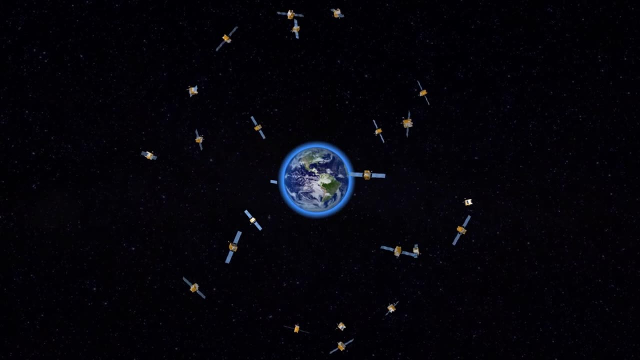 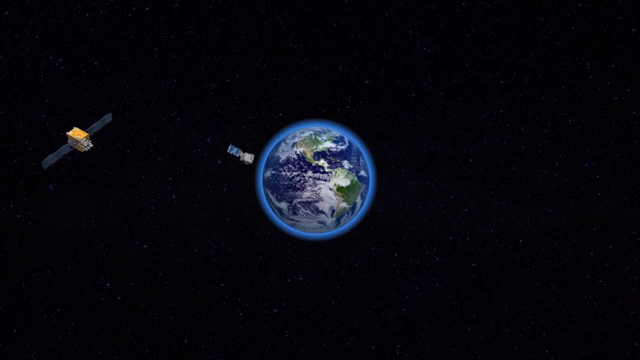 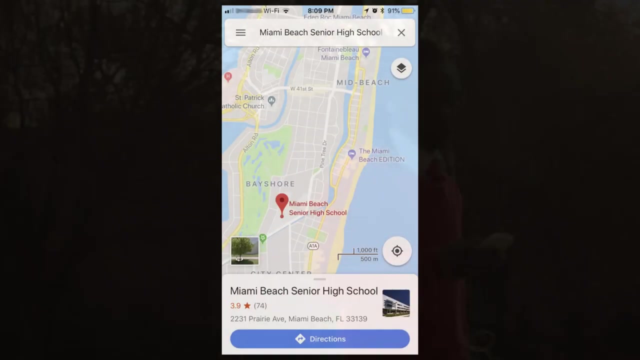 Well, it turns out, COSMIC-2 satellites make use of some other satellites, Ones that were intended for a completely different purpose. GPS satellites circle Earth from very far away, Many times as far away as the COSMIC-2 satellites. These satellites constantly send out the radio signals that your smartphone uses to know exactly where you're located and how to get where you need to go. 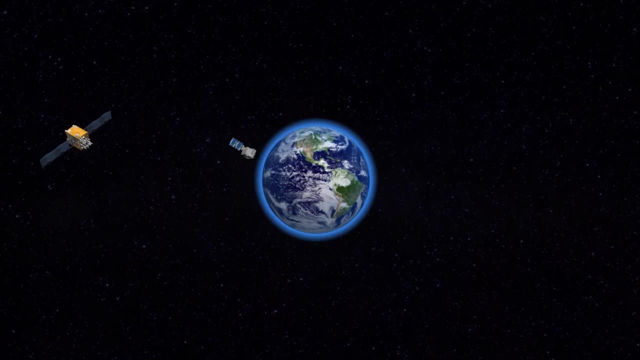 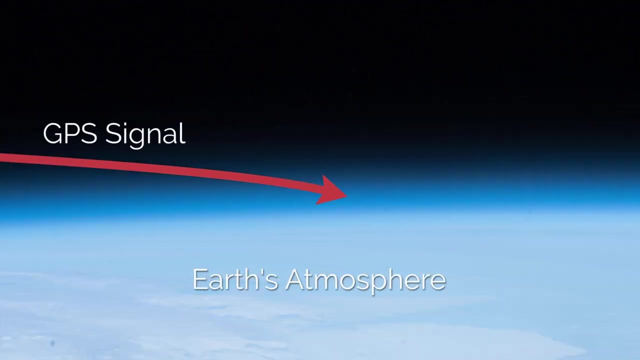 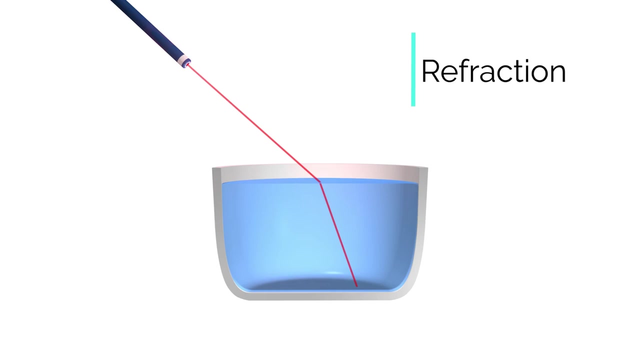 But these radio waves can change your life. They can be used in a very different way. Scientists notice that when the GPS radio waves enter the atmosphere, they bend slightly, Very much like how light bends when it enters water. This is called refraction. 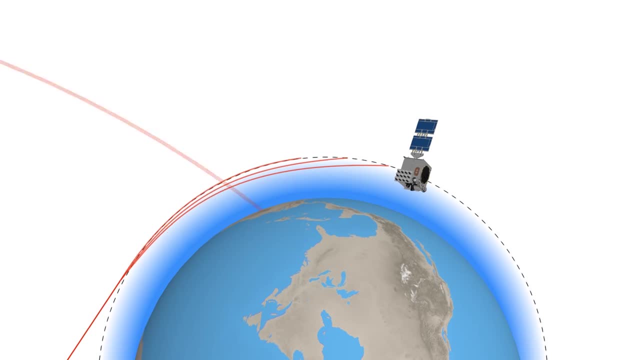 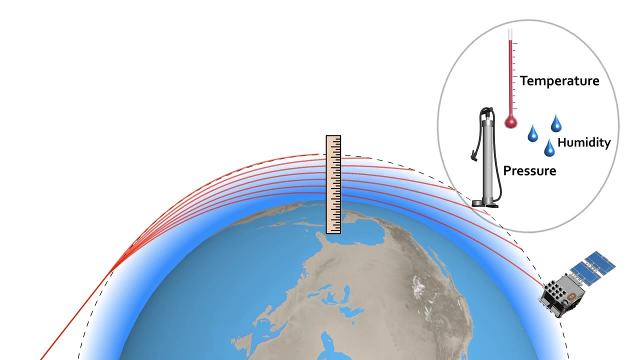 It turns out that by looking at exactly how much the radio waves bend, scientists can get a picture of the temperature, air pressure and humidity in the atmosphere. This is called radio occultation. Data from COSMIC radio occultation helps create more accurate weather forecasts.